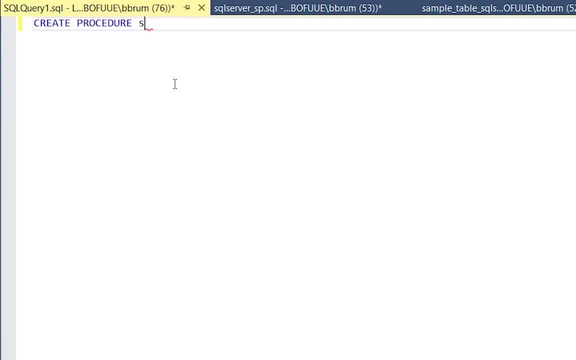 Next, we need to provide a name for our new procedure. Given that we will be selecting data from our newly created customer table, let's call it selectCustomer. We then add the keyword as, which indicates we are about to define what the procedure is. 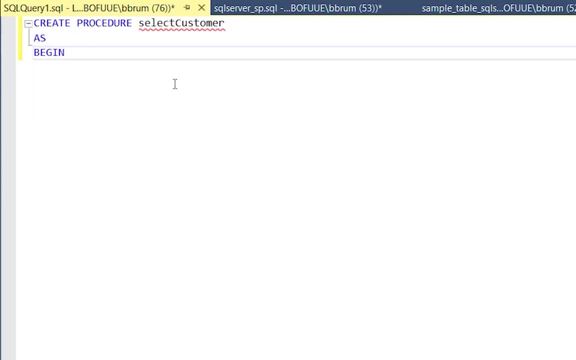 Next we add the word begin. I like to do this on a new line to make it more readable. After the begin keyword we'll leave a gap to add in the code that we want to run. Then we add the end keyword on a new line. Inside the begin and end keyword is where we can add the. 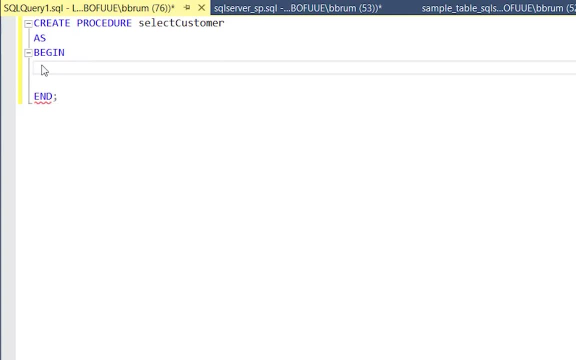 code for the procedure to run. We then add the end keyword on a new line. Inside the begin and end keyword is where we can add the code for the procedure to run. We want to select some data from the customer table, so let's write a query for that. 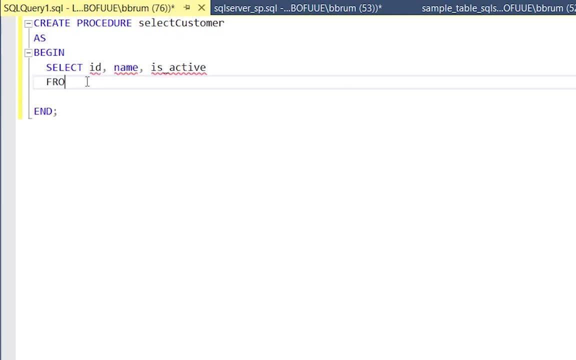 We'll write selectID name is active from customer and add a semicolon. So this is our stored procedure. When we run this create procedure statement, a new procedure is created on the database. Let's run this now If you're using SQL Server. 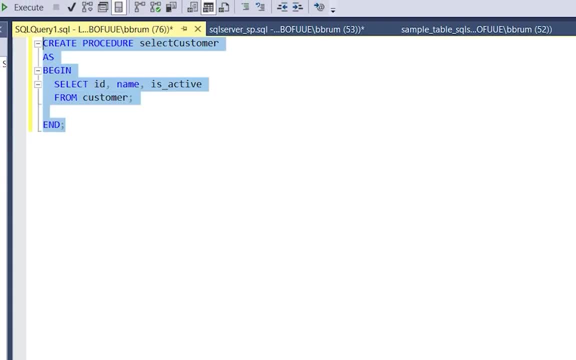 Management Studio. you might see a bunch of red underlines here, but we'll try to run it anyway. Let's run this now. If you're using SQL Server Management Studio, you might see a bunch of red underlines here, but we'll try to run it anyway. 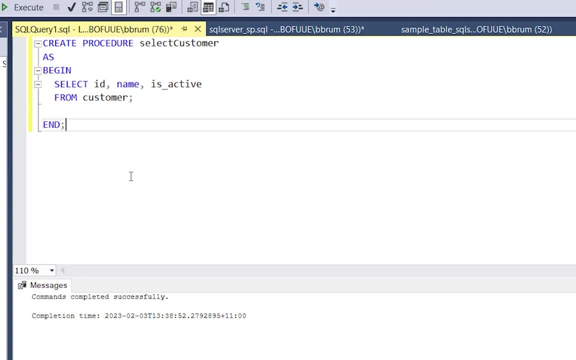 When we run this script, we can see it has been created successfully. Now we have created the stored procedure. the next step is to run it. To do this, we use the exec command or the execute command. I'll use exec because it's shorter. 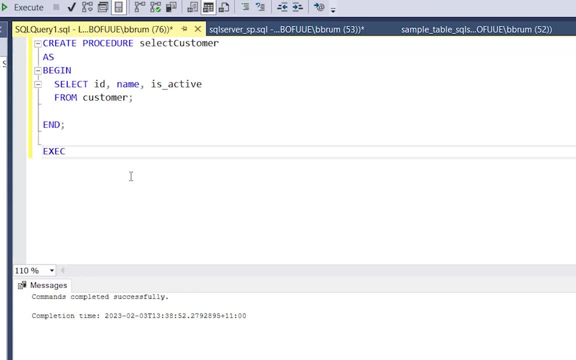 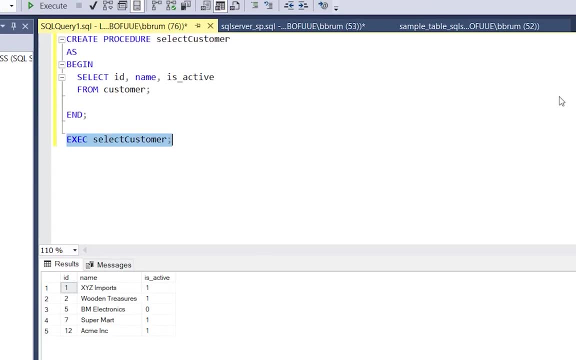 but you can use either one Type exec, then the procedure name, then a semicolon. Run this command, The procedure will be run. You'll see the results at the bottom of the window. It looks just like the results of a select query. This is because our stored procedure ran a select. 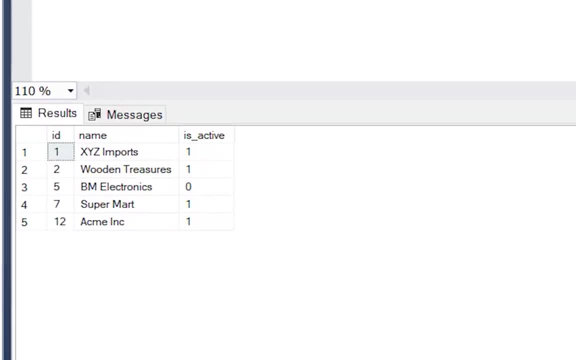 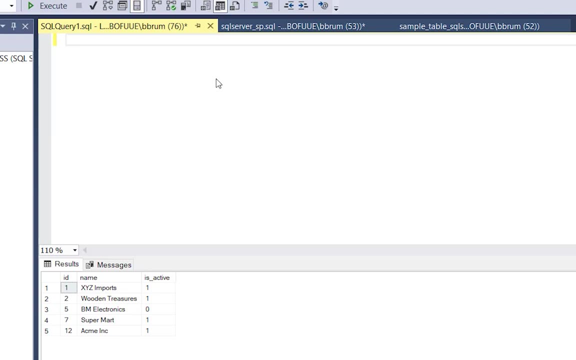 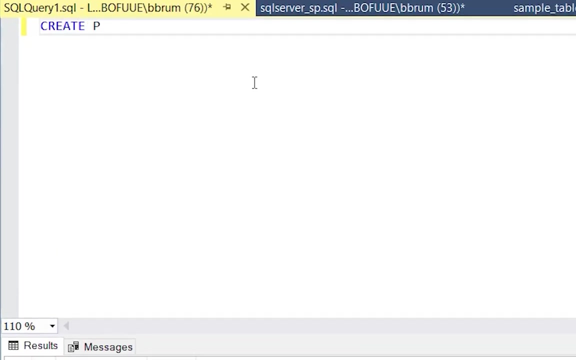 query inside it. So that's how you can create a simple stored procedure to select data. Let's see a few more examples. Now we will create a stored procedure to insert data. It starts the same way as the first example: We write create procedure, then we give it a name. 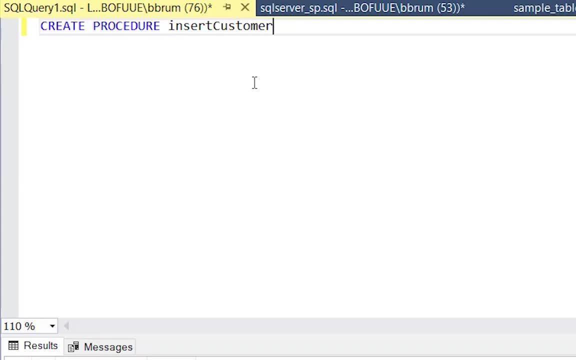 Let's say we want to insert a new customer record with this procedure, so we can call it insert customer. We then have the begin on a new line and the end on a few lines below that. What do we put inside our procedure? We want to add an insert statement here, so we enter insert into: 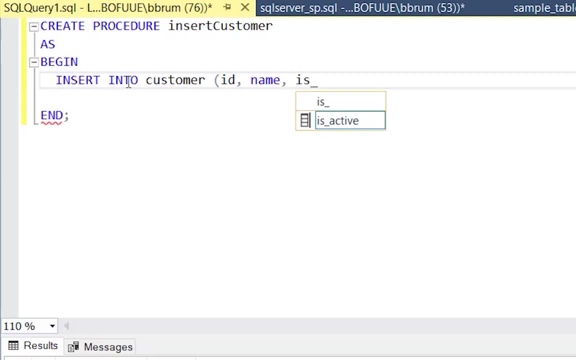 customer then specify the columns which are id name and is active. We then specify values. After the bracket is where we add in the values we want to insert. But what do we insert? How do we enter the values we want to insert? This is where parameters can be used. A parameter is an. 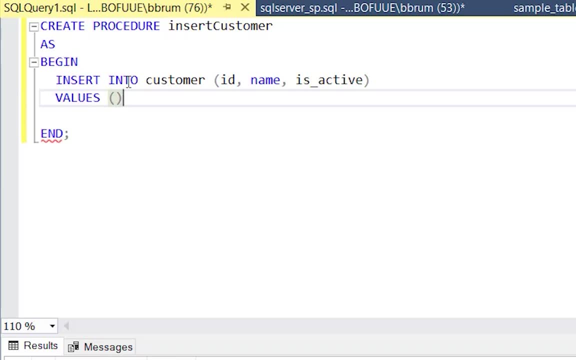 input to a stored procedure that is used within the code in the stored procedure. The input to a stored procedure is used within the code in the stored procedure. The value is provided when the procedure is run. For us, this means that we can provide the. 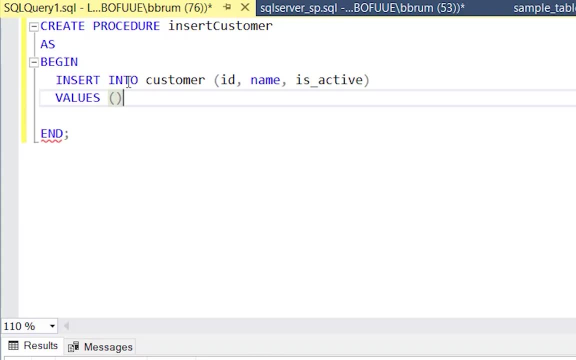 values for the insert statement as parameters when we run the procedure. To do this, let's add one parameter. We add a parameter by adding brackets after the name of the procedure. Inside the brackets we specify a few things. First, we add the at symbol. This indicates that this is a 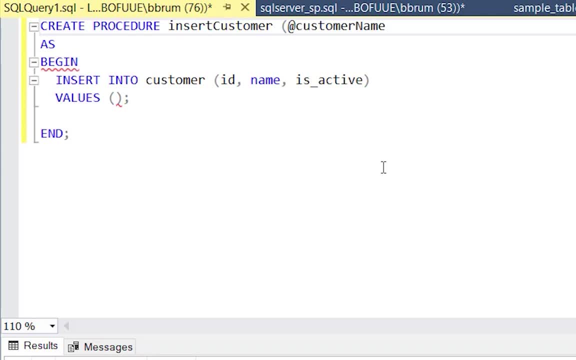 parameter. We'll call ours customer name, just so we don't get it confused with the name column in the table. Finally, we have the data type. This is a name of the customer, So we'll give it a VAR chart type and a length that matches the name column of 100.. We close the brackets. 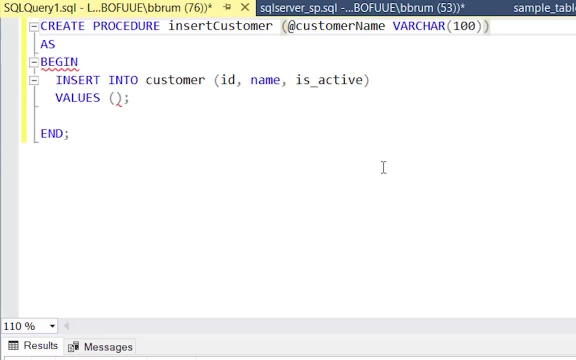 before the begin keyword. Now we have specified a parameter. we can use this in our insert statement For the id column. ideally we would have this auto-generated or provided as a parameter, But to keep it simple, for now we'll just add a static value of 4.. 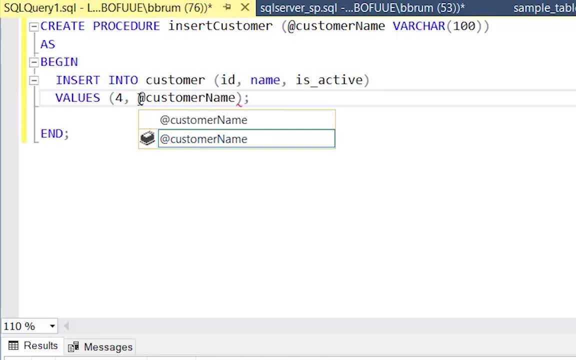 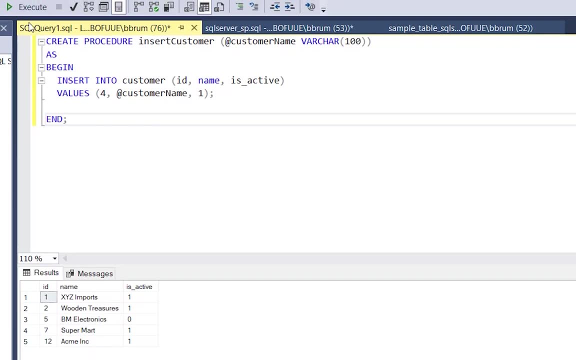 we specify the name of the parameter, which was customer name For the isActive. we can set that to 1.. Now our procedure is complete. We can run this script and the procedure is created, If you see some red lines here or try to run the query. 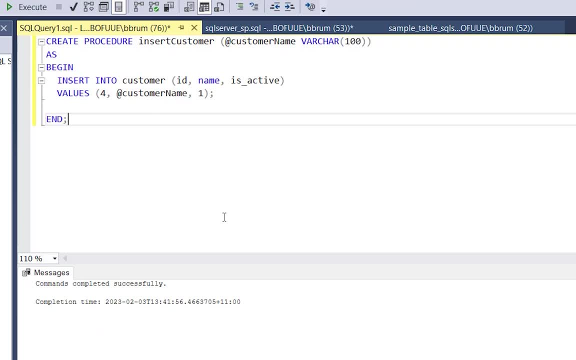 and get an error about the code being the only statement in the batch. this is because SQL Server expects you to end the batch of statements before running another one in the same script. If this was a single script, you could add a forward slash character to end the batch, or we could just select the statement we 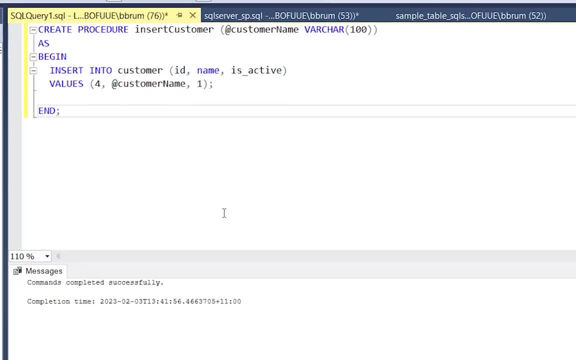 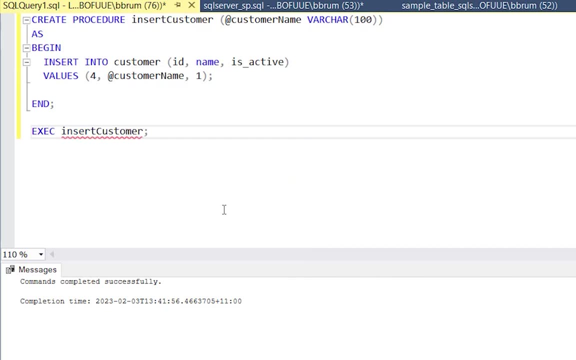 are running and run that which should work. Let's call this stored procedure. now We can write an exec statement, then the name of the procedure. Let's run this command When we do. we get this error here. What happened? This error is shown. 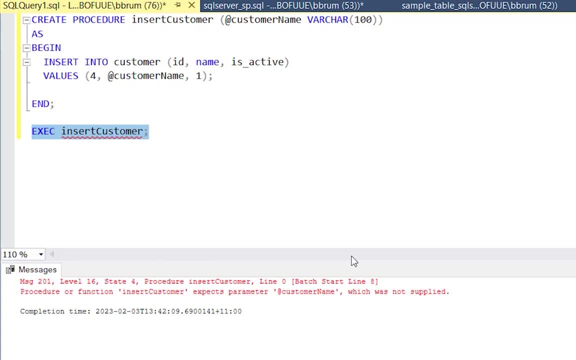 because we ran the stored procedure that expected a parameter but we did not provide a parameter. Let's fix that. To add a parameter when calling a procedure, we add a space after that The procedure name. Next we specify the value to use for the parameter, Because 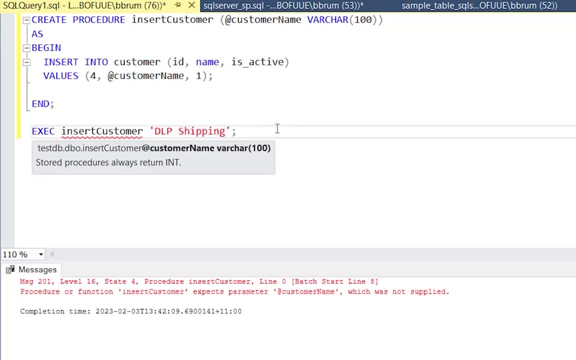 it's a string, we enclose it in quotes. We don't enclose this in brackets like in some other languages. We just have a space and then the parameters. Now we can run the command again. We can see here: the command is successful. It shows a. 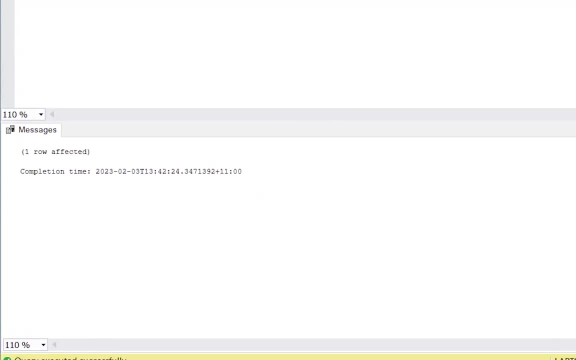 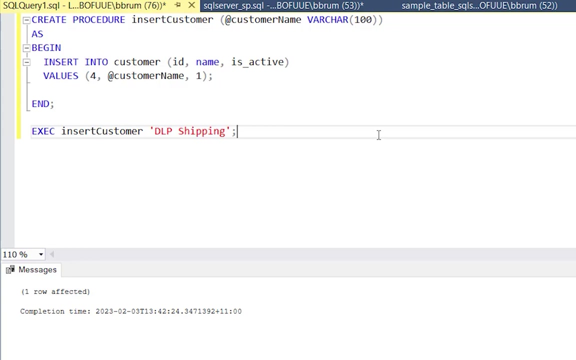 green tick and says one row is affected. There is no select output shown because the procedure did not include any select statements. We can run a select query here, just a simple one, and we can see the results. We can see our new value is inserted into the table. So that's how you can create a procedure. 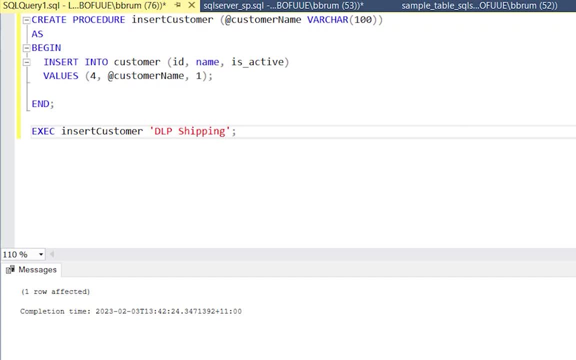 that inserts data. There's a whole lot of logic you could and should add to a procedure like this, but that's the basic version. What else can you do? Let's see an example of a stored procedure that updates some data. We start with the same. 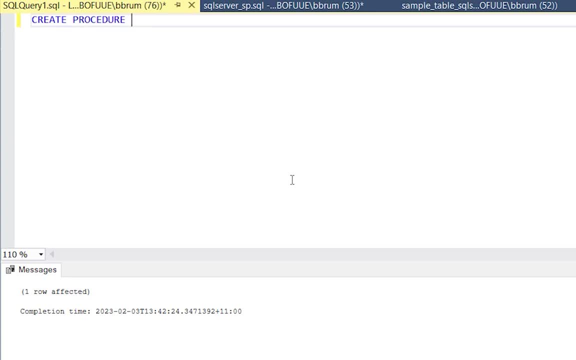 structure as the previous example with the create procedure statement. We'll call it updateCustomer. We'll call it updateCustomer. We'll call it updateCustomer. What parameters do we need? We need to know two things when we are updating a record: What the new value should be and what the criteria is for the rows to. 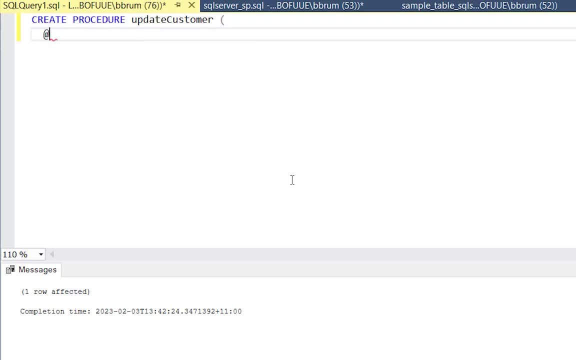 update. Let's say we want to update the customer name, so the new customer name value is one parameter. And let's say we want to work out which customer to update based on the ID, so that will be our second parameter. We separate them in. 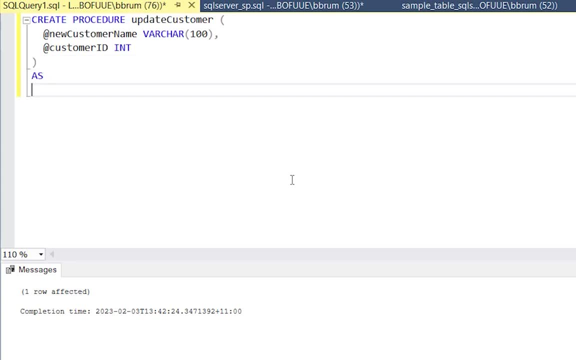 the parameter section here with a comma. We've separated them onto different lines to make it a little easier to understand. We'll call it updateCustomer. Our procedure can be a little easier to read. Inside our procedure we write our update statement. This update statement will update the customer name to the value provided as. 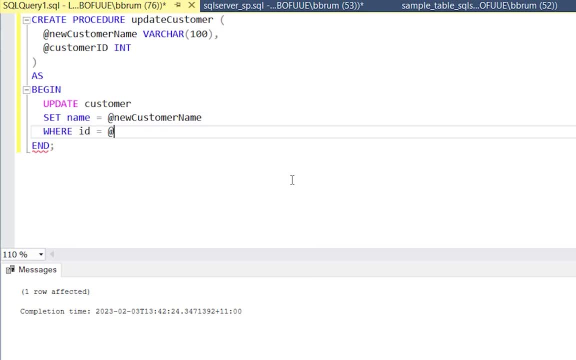 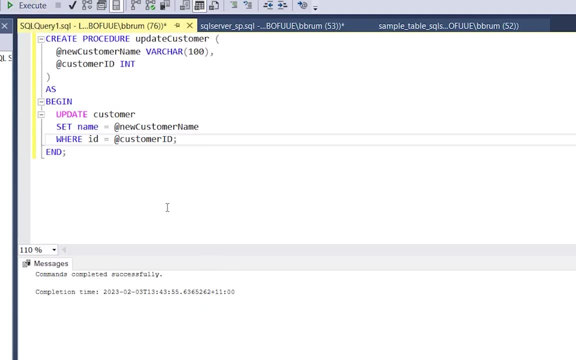 a parameter. The where clause will allow us to update only the customer records with the provided ID. Our procedure is now written. We can run this script and the procedure is created. Now let's call it. We can call it in the same way as the other procedures. 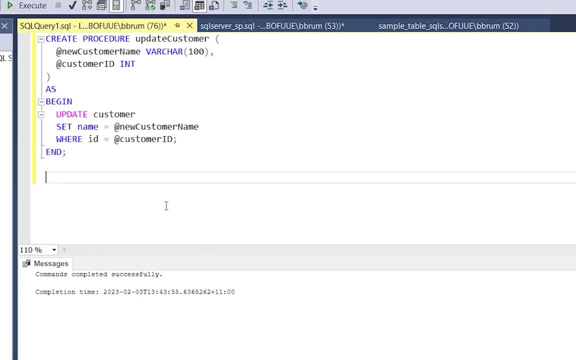 This procedure is a little different, as we have two parameters. We add both parameters separated by a comma. We have a name of abcexports and an id of 2.. We can run this statement and can see it was successful. How can we see what the data looks like? 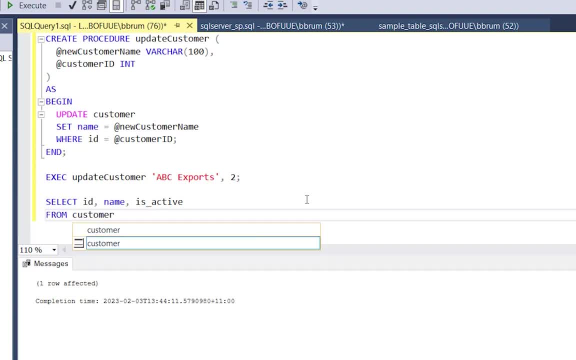 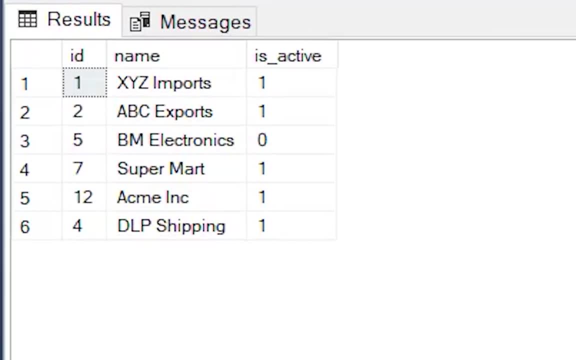 We can run a select query. We'll run the same one as before to see all the data in one table. In our results we can see that the record we specified in the update procedure has the new value we specified. The record with an id of 2 now has a name of abcexports. 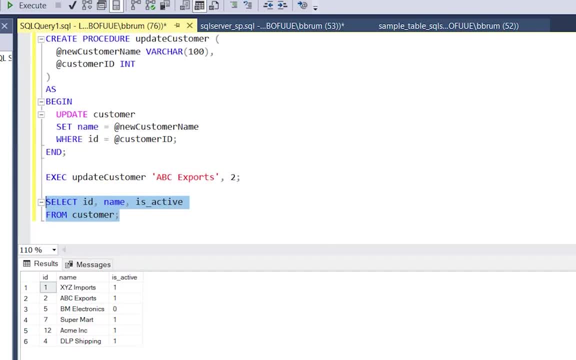 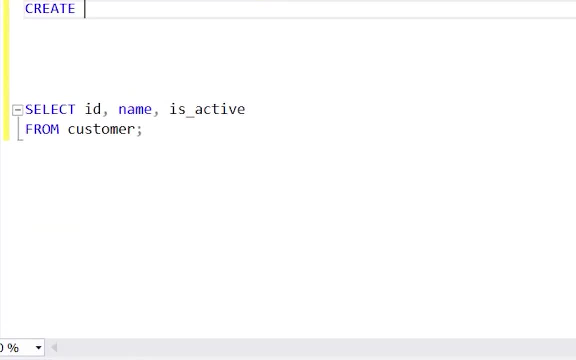 The final example we'll cover is how to delete a row in a stored procedure. It works in the same way as other procedures. We'll start with an empty procedure like this, which we've called deleteCustomer. To delete a row, we need to know the criteria for the row to be deleted. 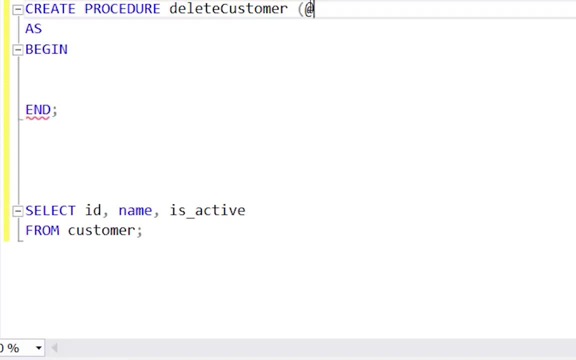 Let's say we want to specify an id and delete that row, So we add that as a parameter. Now inside our table we can see that we have an id of 2.. To specify our procedure, we write a delete statement. 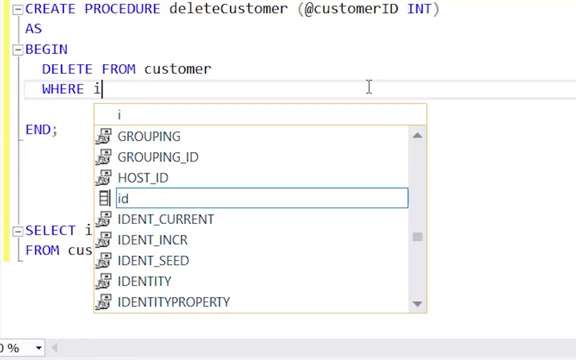 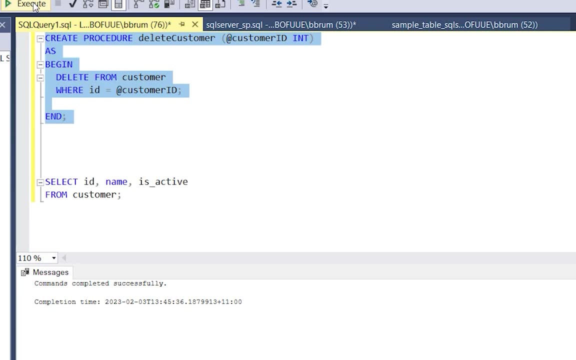 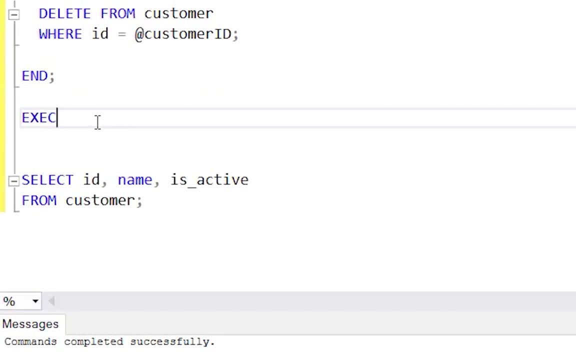 We delete from our customer table and add a where clause that deletes based on the id parameter. The procedure is now written. Let's run the script and the procedure is created. Let's run the procedure. We can run it in a similar way to the other procedures, using the exec statement. 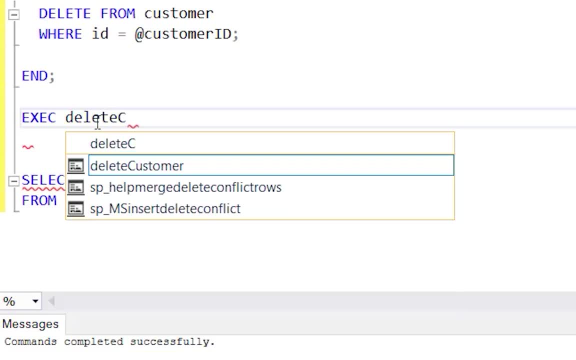 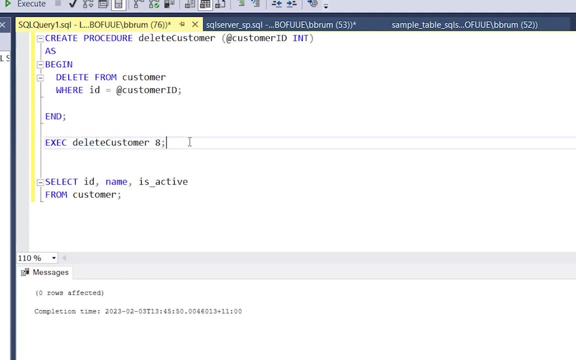 We specify a parameter here. In this example we'll provide an id for a row that does not exist. just to see what happens When we run this command. we can see the procedure runs. There are no errors, but in the output panel in SSMS it shows us that zero rows were affected. 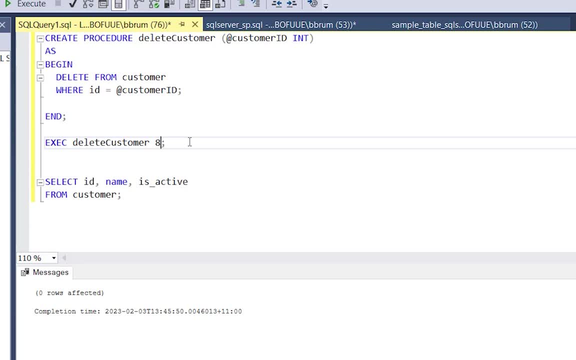 This indicates that no rows were deleted. Let's call the procedure again, but we'll use an id for a record that exists. We get the same success message, but the response says that one row was deleted. Now we'll run a select query to see the data. 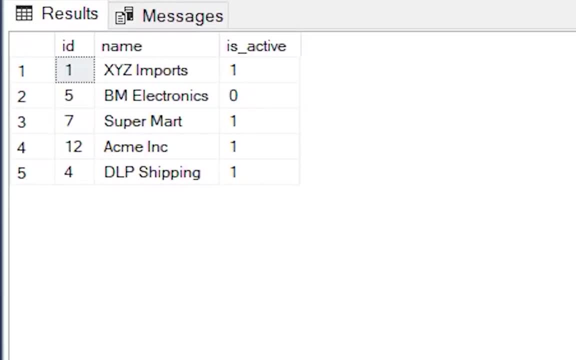 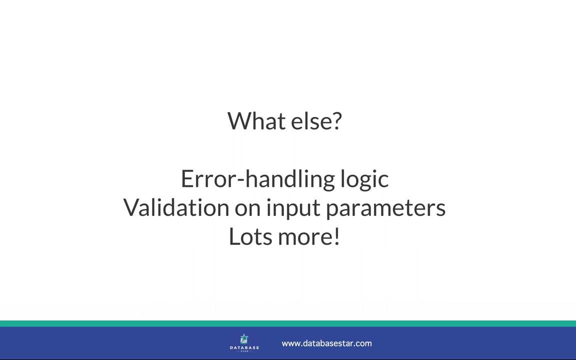 We can see the results here and see that the id we specified is no longer found in the table. This means our delete statement is successful. So we've seen some basic examples of stored procedures in SQL Server. What else can you do? You may want to add some error handling logic to your procedure, such as checking if a row